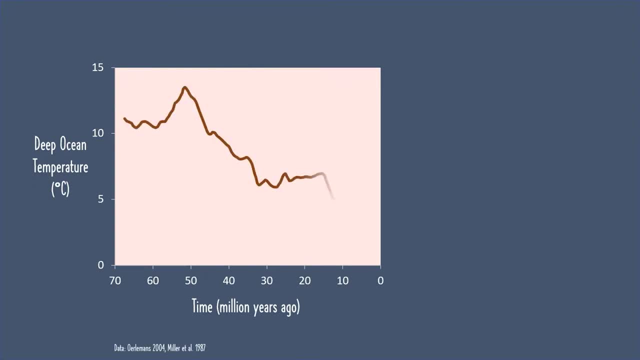 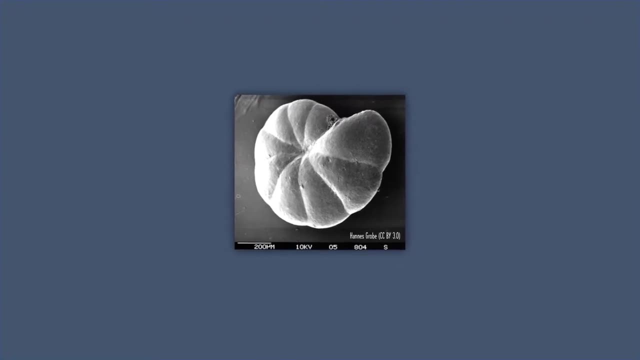 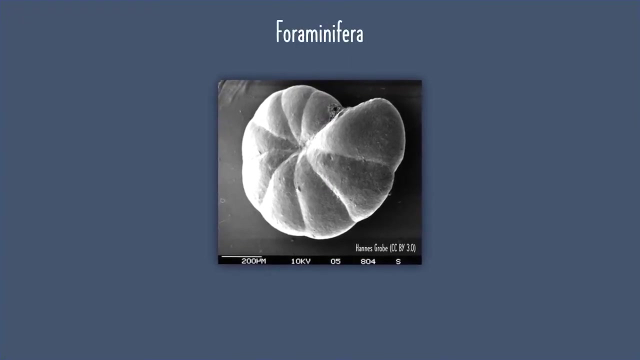 millions of years ago by doing chemical analysis of the fossilized shells of tiny organisms that lived at the bottom of the ocean. This image, taken under a microscope, shows one of these creatures. It's a type of organism called foraminifera. 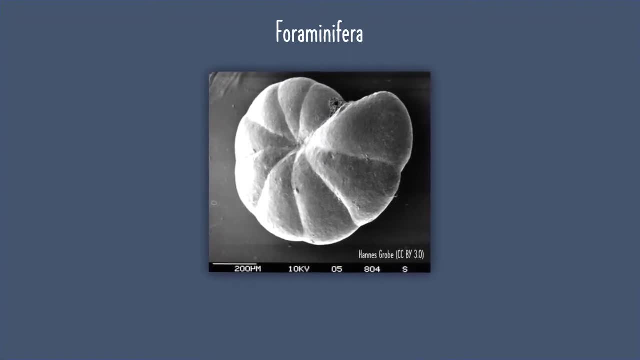 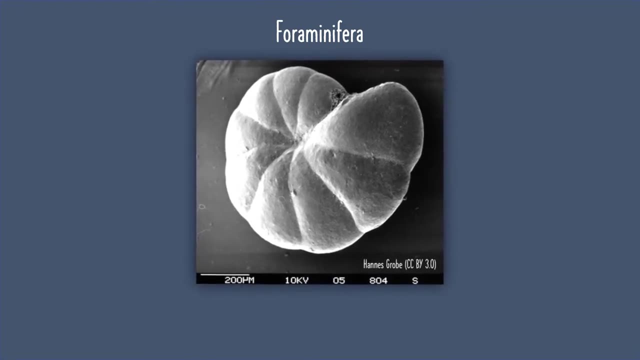 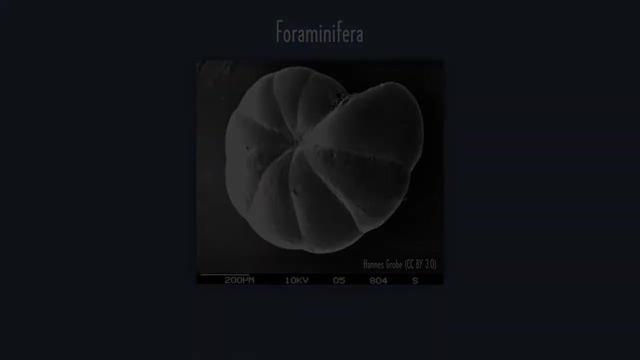 and it's less than a millimeter wide. How can something so small tell us about things so vast as the ocean or giant ice sheets? As background to answering that question, we need to understand a little bit about the chemistry of atoms. Chemical elements such as oxygen and carbon have different isotopes—forms of the atom. 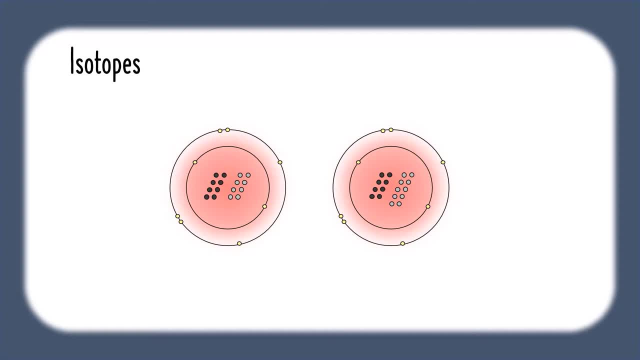 that have the same number of protons but different numbers of neutrons. For example, two isotopes of oxygen are oxygen-16, with 8 protons and 8 neutrons, and oxygen-18, with 8 protons and 10 neutrons. Oxygen-18 atoms are heavier than oxygen-16 atoms because they 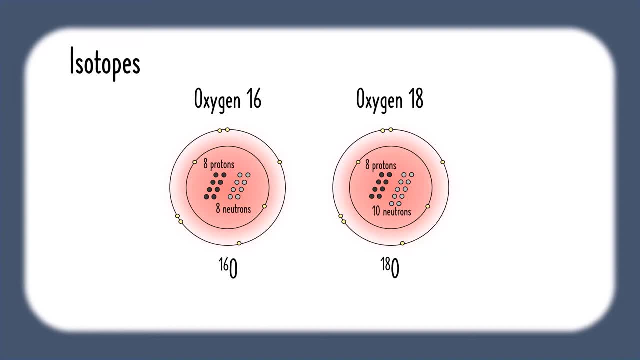 have more neutrons. These two isotopes are both stable, meaning that they don't undergo radioactive decay. As a result, a stable oxygen isotope that existed in the ocean hundreds of millions of years ago will have a stable, stable, stable, stable, stable, stable, stable. 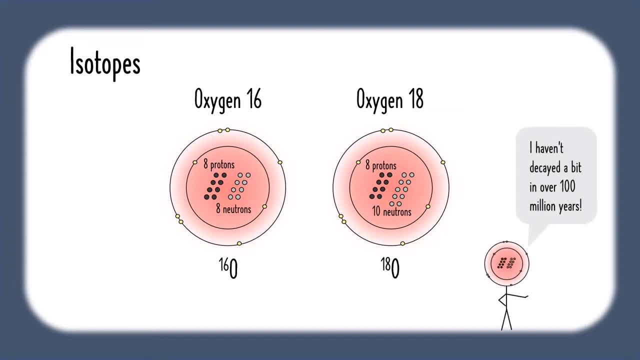 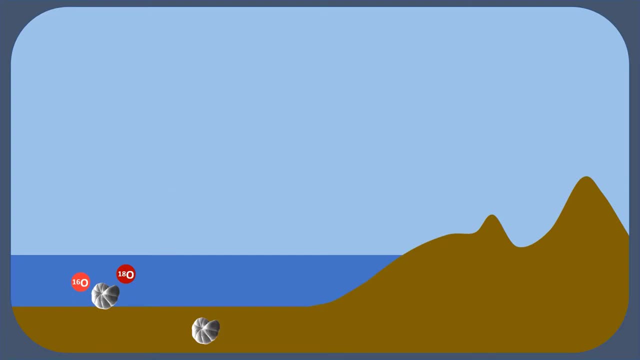 to the Earth's temperature. This is how it works At the ocean surface. lighter isotopes evaporate more easily from seawater than do heavier ones. The water vapor containing light isotopes then gets transported in the air and eventually condenses During times when. 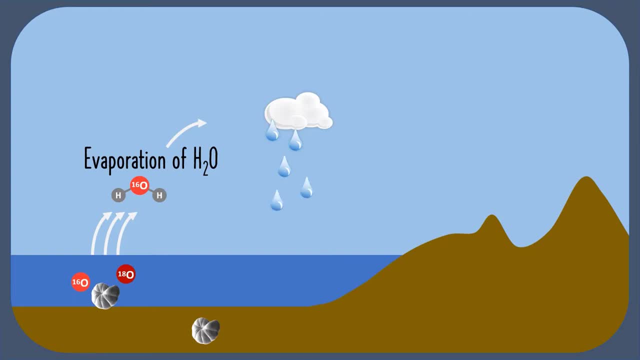 the Earth is warm, the condensed water vapor falls back towards the Earth as rain, either over the ocean or over land. If over land, the water eventually drains back to the ocean, and when the ocean is cold, some of the condensed water falls on top of ice sheets and glaciers.